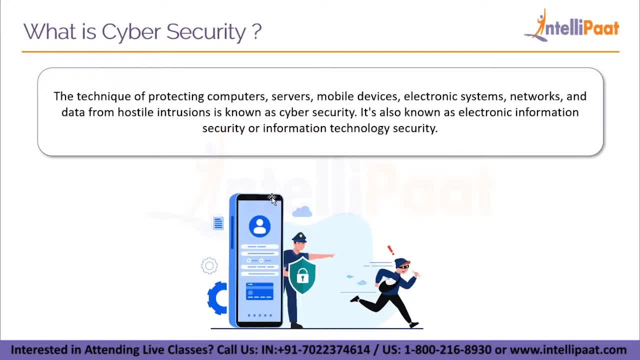 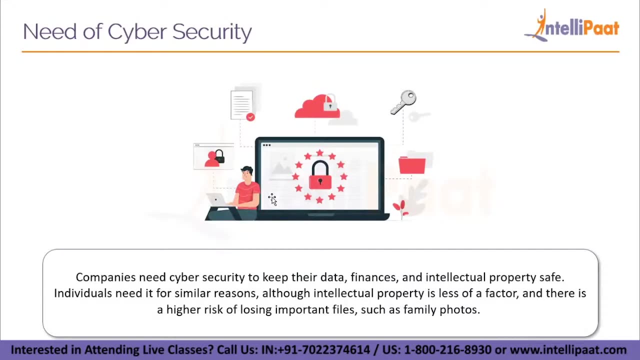 And this is known as cyber security. It is also known as electronic information security or information technology security, IT security in short. Now let us take a look at the need for cyber security. Companies need cyber security to keep their data, finances and intellectual property safe. 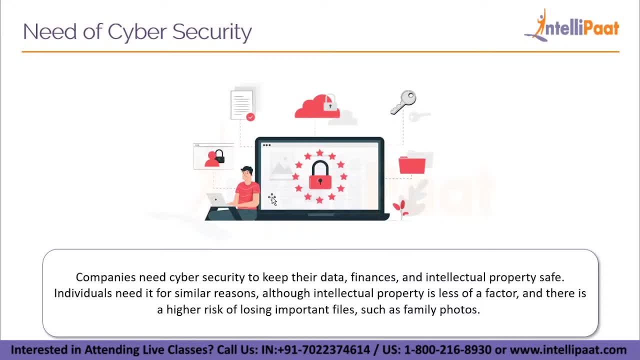 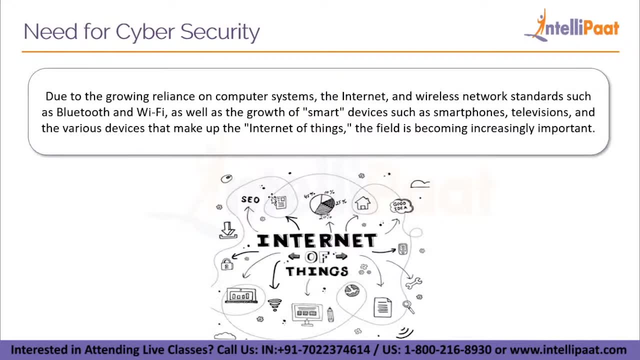 People need it for similar reasons. Although the intellectual property is less of a factor, there is a higher risk of losing important files such as family photos. Due to the growing reliance on computer systems, the internet and the wireless network standards such as Bluetooth and Wi-Fi, as well as the growth of smart devices like smartphones, televisions and the various devices that make up the internet of things, this cyber security field is becoming increasingly important. 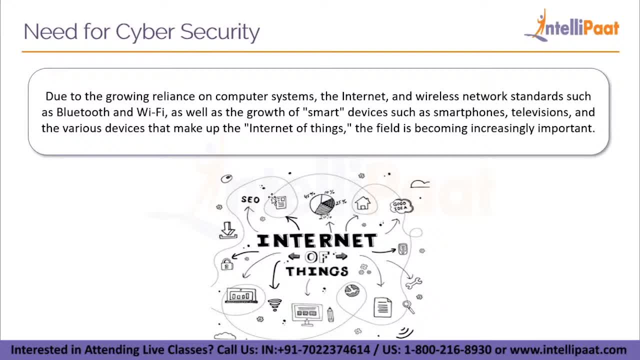 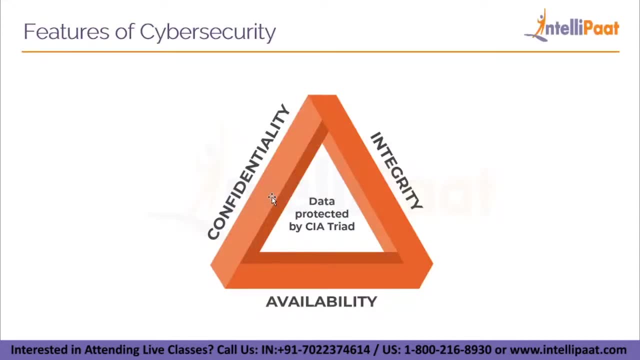 is as essential as electricity and water in present times, there are people who try to misuse this, so cyber security will always have a demand. now let us move on to the features of cyber security. the core underpinning of the information security domain is the cia triad. these features: 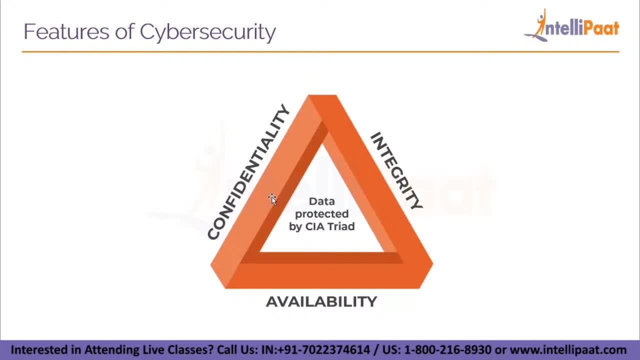 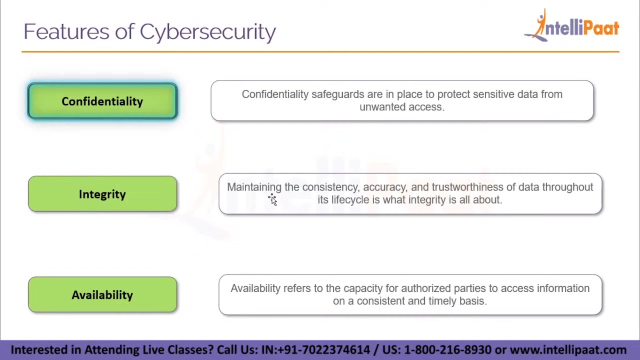 are confidentiality, integrity and availability. every security control and every security vulnerability can be viewed in light of one or more of these concepts. for a security program to be considered comprehensive and complete, it must adequately address the entire cia triad. now let us briefly know about these features. confidentiality: confidentiality: safeguards are in place to protect. 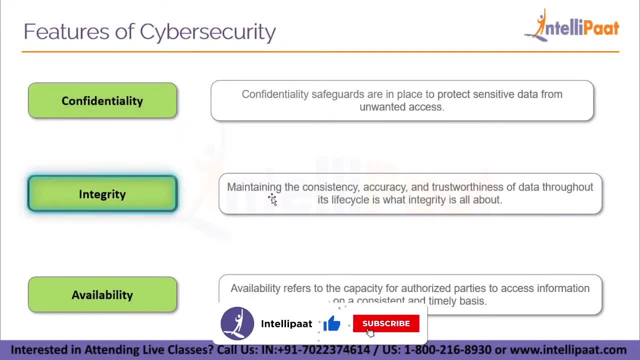 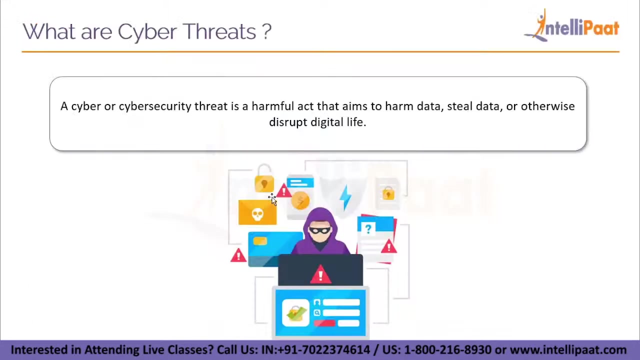 sensitive data from unwanted access. integrity: maintaining the consistency, accuracy and trustworthiness of data throughout its life cycle is what integrity is all about. availability: availability refers to the capacity for authorized parties to access information on a consistent and timely basis. now let us move on to what are cyber threats? a cyber 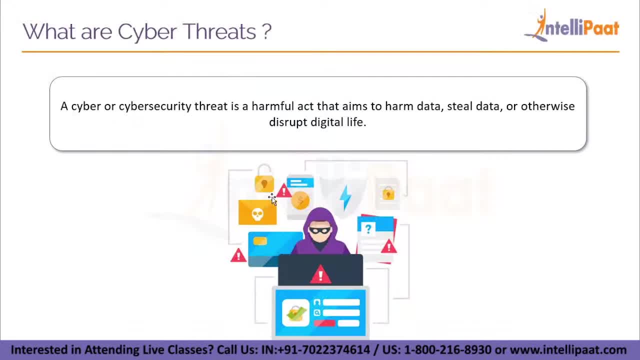 or cyber security threat, is a harmful act that aims to harm data, steal data or otherwise disrupt digital life. it can be called an event that has the potential to negatively affect an organization's operations. so it- cyber threat, can basically cause economical harm to an organization or completely shut down an 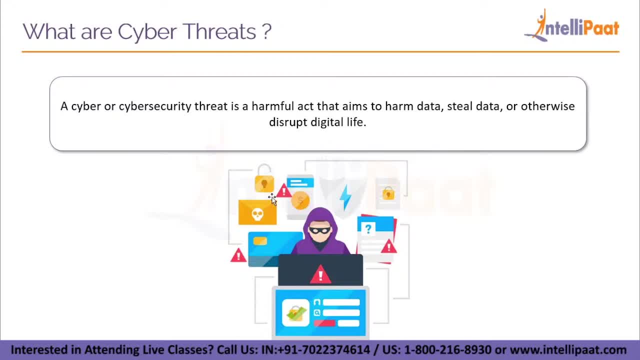 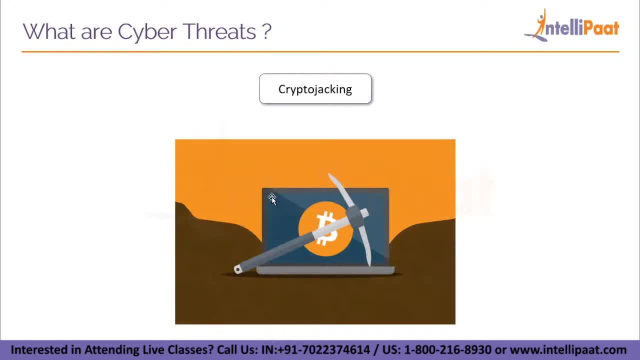 organization's operations for a day or a week or whatever time period that might be. so one example of a new kind of cyber threat in recent times is crypto jacking. the cryptocurrency movement also affects cyber security in other ways. for example, crypto jacking is a trend that involves cyber. 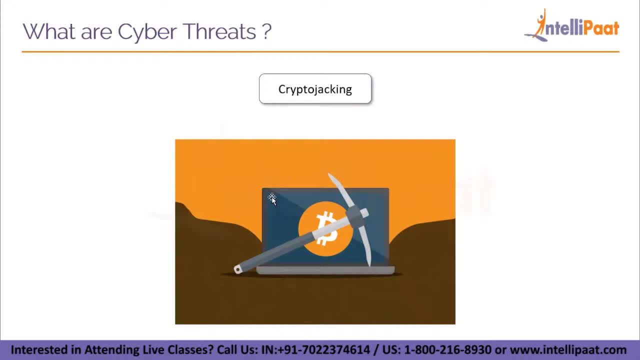 criminals hijacking third-party home or work computers to mine these cryptocurrencies, because mining for cryptocurrencies like the bitcoin, for example, requires immense amounts of computer processing power. hackers can make more money by secretly piggy banking on someone else's computers for businesses. crypto jacked systems can cause serious 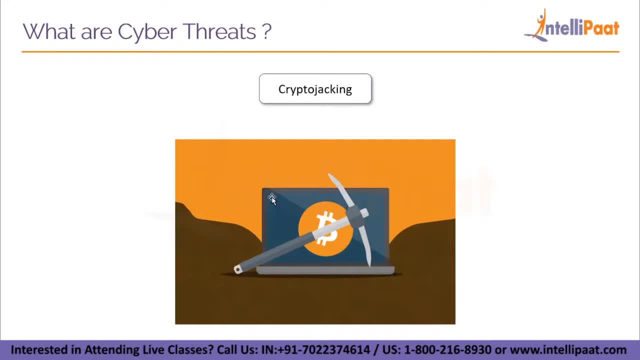 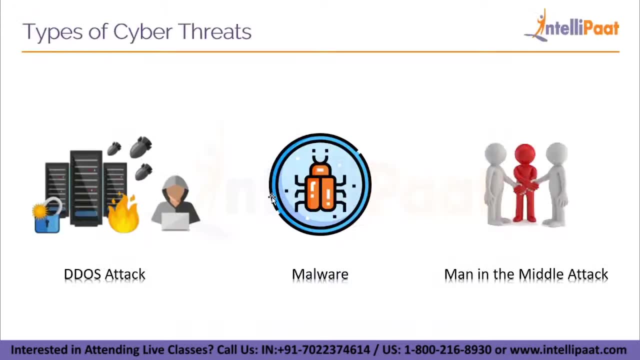 performance issues and costly downtime, as the it department works to track down these and resolve the issue. now let us know some of the common cyber threats. the common cyber threats are ddos or cyber threats are common cyber threats are common cyber threats? are common cyber threats are? 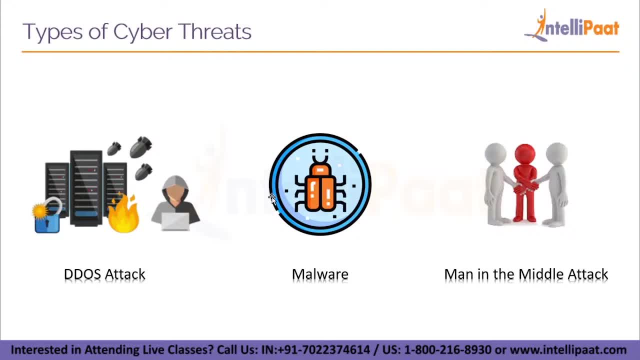 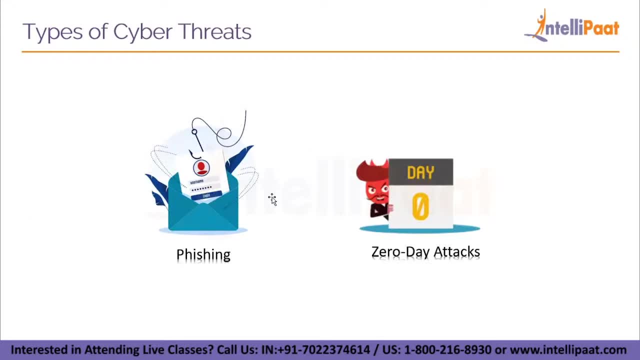 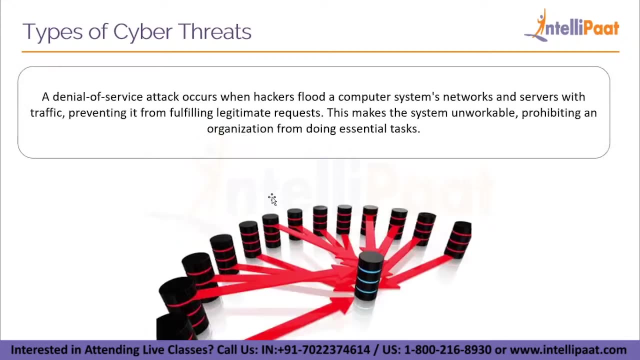 also known as the distributed denial of service attack. we also have malware- and we have man in the middle- attack phishing and zero day attacks. these five are the most common cyber threats. let us take a brief look at all of them. so a denial of service attack occurs when hackers flood a computer system's 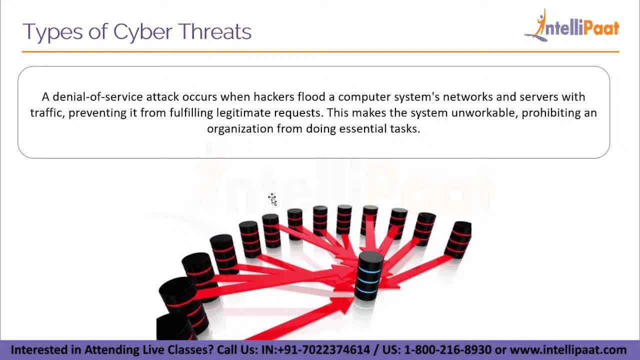 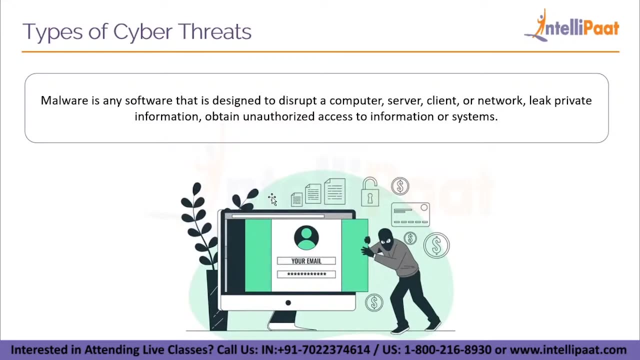 network and servers with traffic preventing it from fulfilling legitimate requests. this makes the system unworkable, prohibiting an organization from doing essential tasks. malware is any software that is designed to disrupt a computer server, client or network, leak private information, obtain unauthorized access to information or systems. there are many types of malware, some of 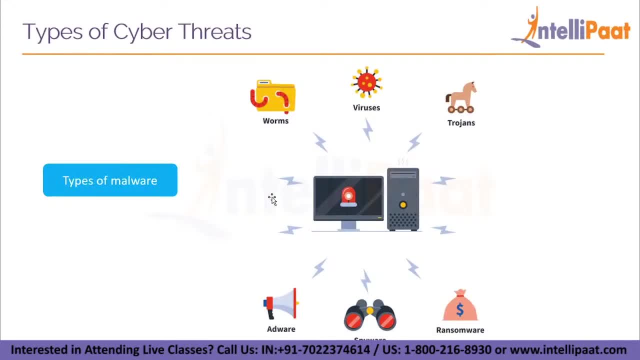 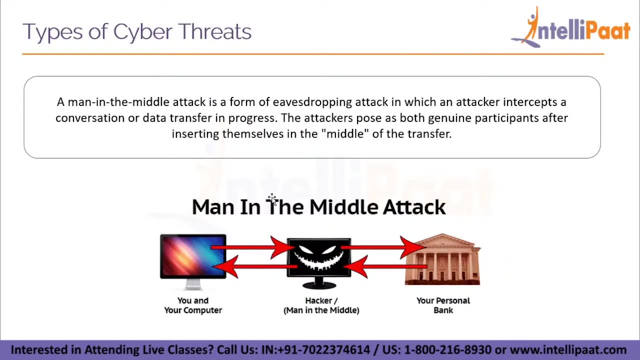 them are worms, viruses, the trojan virus, adwares, spywares and ransomware. man in the middle attack. a man in the middle attack, or also known as mitm attack, is a form of eavesdropping attack in which an attacker intercepts a conversation or data transfer in progress. just a quick info, guys. if 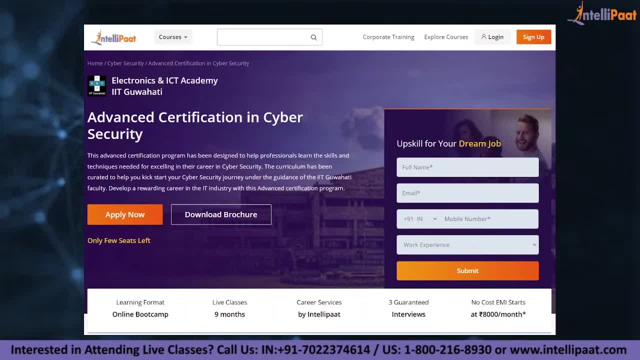 you want to make a career in cyber security, then intellipad provides a advanced certification in cyber security by iit guwahati and it is taught by iit guwahati professors and industry experts. this course is designed to upskill and land your dream in cyber security and it is taught by iit guwahati. 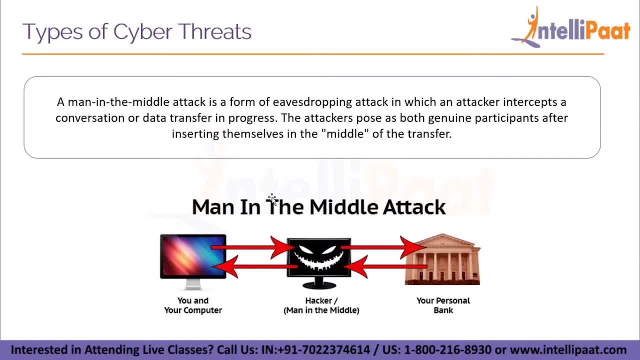 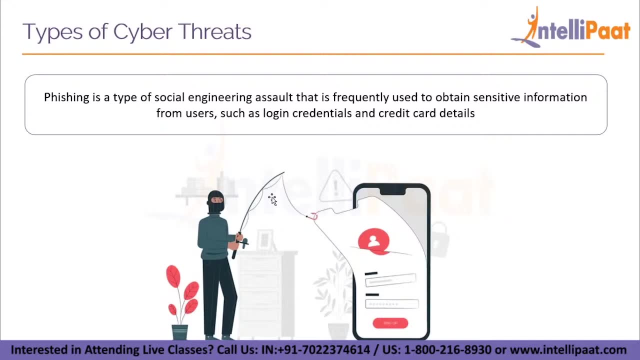 professors and industry experts. now let's continue with the session. the attackers pose as both genuine participants after inserting themselves in the middle of the transfer, that is, they get in between you and your computer and whoever you're talking to. phishing is a type of social engineering assault that is frequently used to obtain sensitive information from users such as. 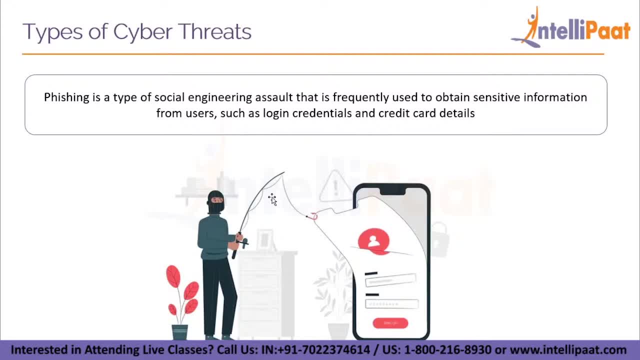 login credentials and credit card details, so these people will basically code an entire ui page. that is a type of social engineering assault that is frequently used to obtain sensitive information. that looks exactly similar like a bank's page or an e-commerce page. so whenever you enter your 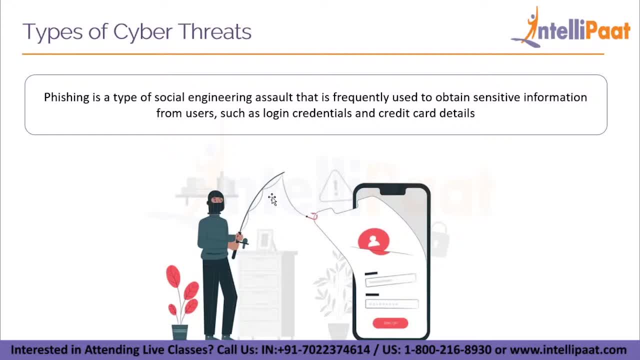 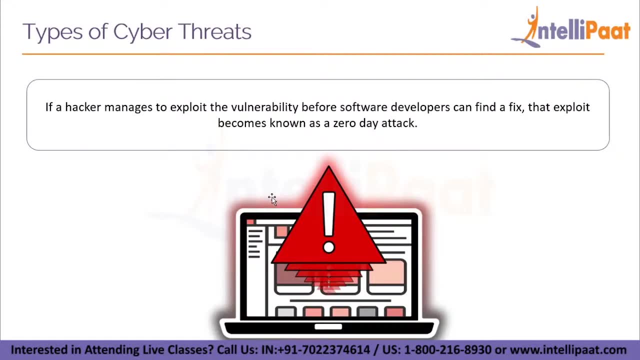 credentials, that is, your username and password of your bank account. they will have access to it and they might transfer funds from your account to theirs. now, last but not the least, let us know about the zero day attack, if a hacker manages to exploit the vulnerability before software. 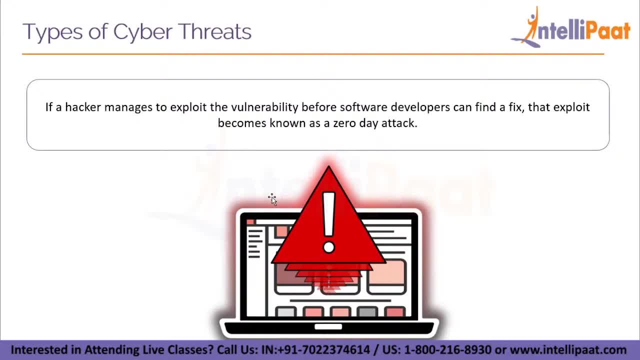 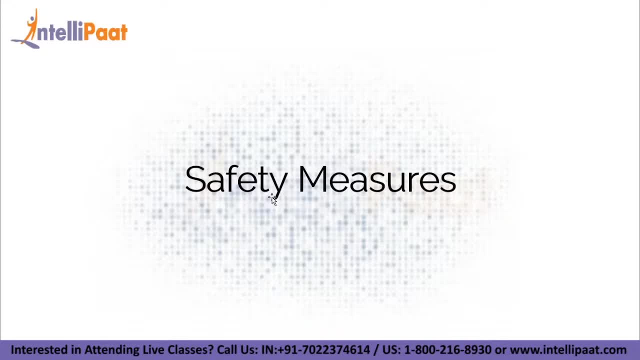 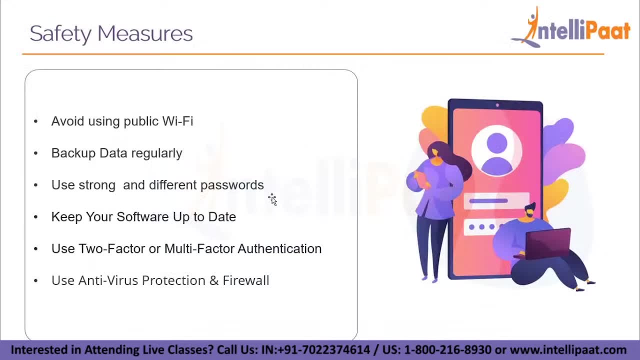 developers can find a bug or a fix. that exploit becomes known as a zero day attack. so now, as we are aware of the threats, let us know how to keep ourselves safe from these attacks. avoid using unprotected public wi-fi on your devices, if at all, or if possible. it can render 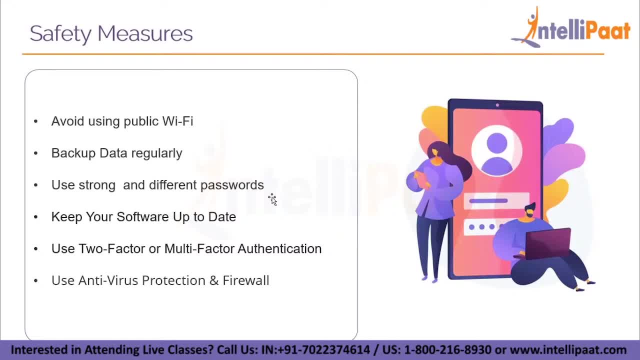 you vulnerable to explorative techniques if you use them. if you must use it, avoid inputting sensitive information on any website, such as your social security number or bank information. when you're not at home, use a vpn or a virtual private network, as it is called to. 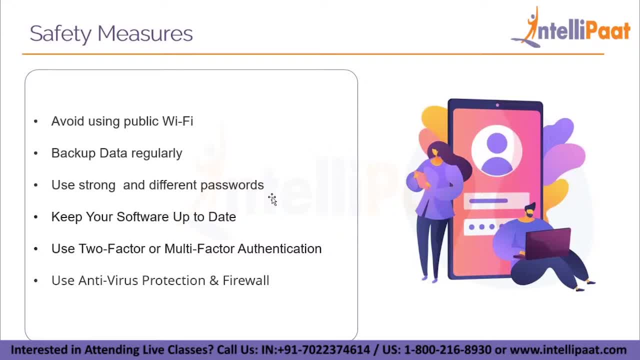 perform your browsing. so this will basically keep you protected from the world wide web and it makes you more difficult to intercept. and the next safety measure is backing up your data. you may have certain types of security breaches less problematic by backing up your data. it won't be. 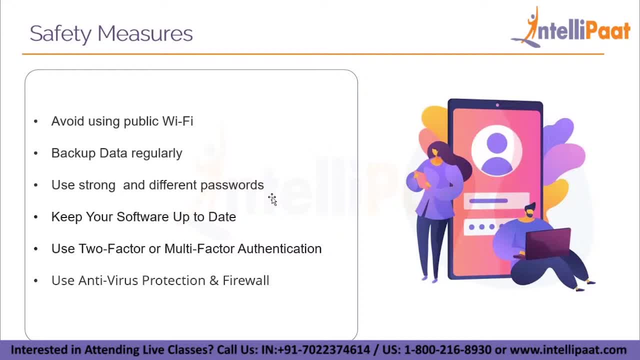 a big concern if a hacker encrypts your data and demands a ransom to decrypt it, if you backed it up a week ago or whenever it might be. so the next safety measure is not to use the same password for everything. it can be risky to use the same password for everything once a hacker has your 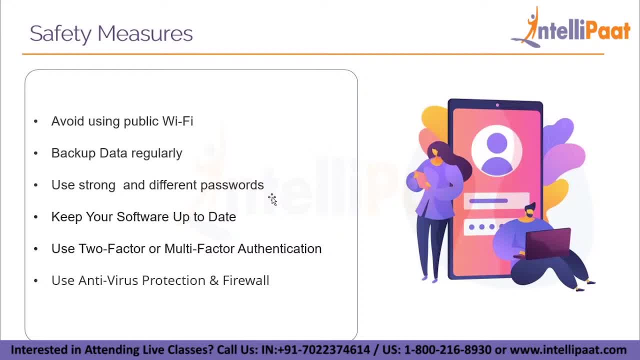 password, they will have access to basically your entire system, as well as any applications that you use. having separate password for each application you use is a great way to improve your security, and changing them frequently will keep you safe from both external and internal dangers. so the next safety measure is keeping your software up to date. cyber attacks frequently. 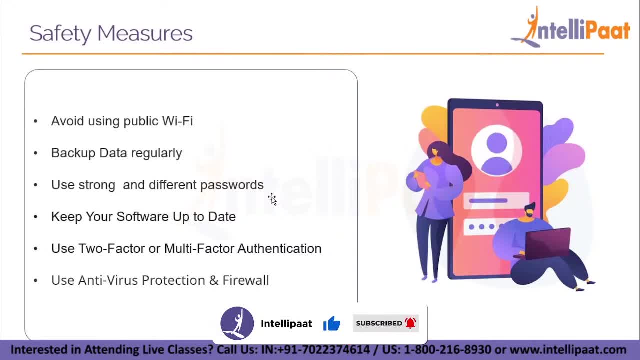 occur because your system or software are out of the current and exposing vulnerabilities. hackers take advantage of these flaws and cyber criminals take advantage of them to get access to your network. it is sometimes too late to take precautionary measures after they have gotten in. to combat this, it is always a good idea. 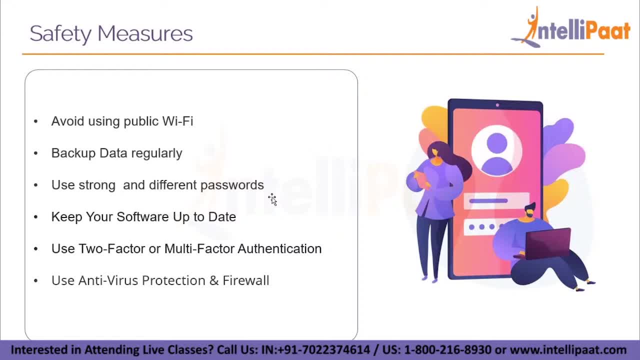 to invest in a patch management system that will keep track of all your software and system upgrades, ensuring that your system is secure and up to date. so the next safety measure is to use either the two factor authentication or multi-factor authentication. so, after you have logged in with your username and 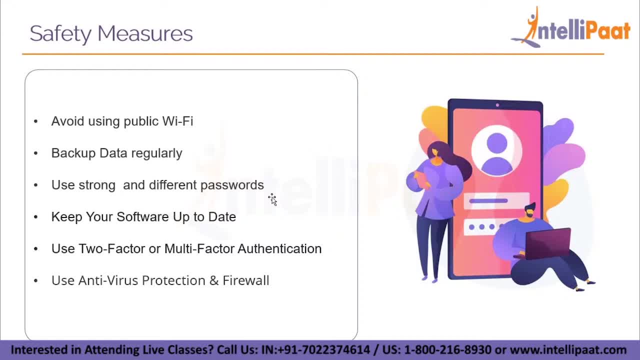 password. that is also called as a single factor authentication- uh, you need to prove your identity. in some situations you will be requiring to input a code given to your phone that is an otp. so username and password becomes your first layer of authentication and your phone otp becomes your. 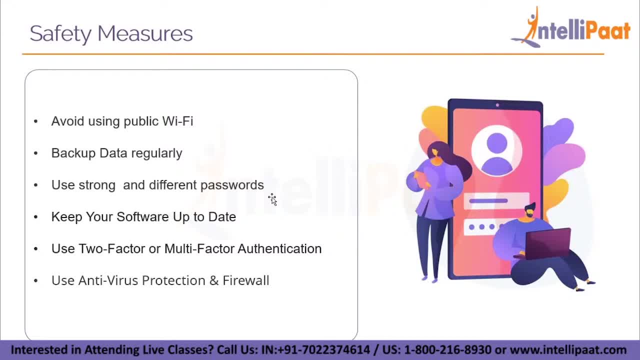 second layer, which is also called as a two-factor authentication. so we have many alternative authentications apart from password. So make sure your authentication is multi layered so that it is hard for hackers to break into your system. And lastly, the safety measure is to use antivirus protection. 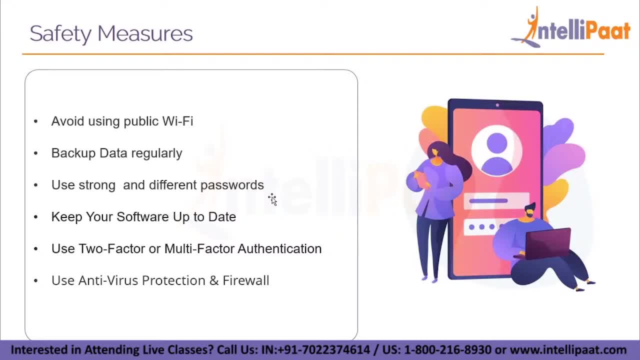 and firewalls. One of the most effective strategies to defend yourself against any cyber assault is to put your network behind a firewall and an antivirus. Any brute force attacks on your network or your system will be blocked by a firewall system before they can cause any. 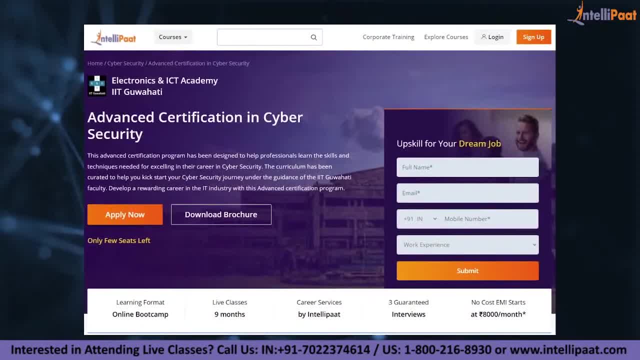 damage. Thank you for watching till the end, guys. Just a quick info, guys, if you want to make a career in cyber security, then Intellipaat provides an advanced certification in cyber security by IIT Guwahati and it is taught.